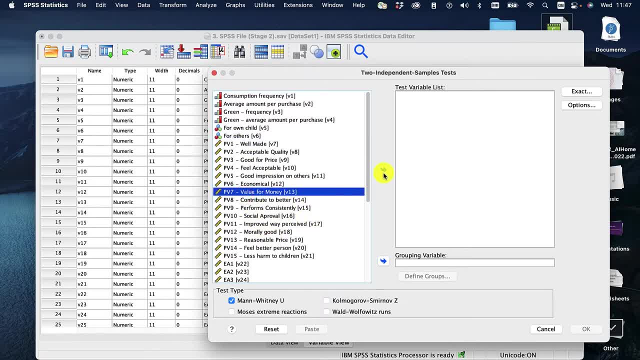 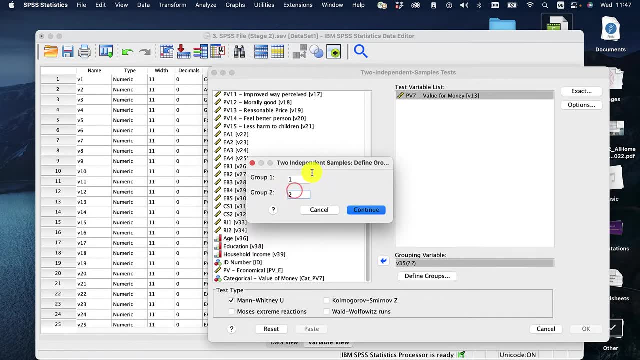 to put in just value for money to make life nice and simple. And the grouping variable I've got is gender. So I'm going to define the groups as 1 and 2, because I know that male is 1 and female is 2.. We might have 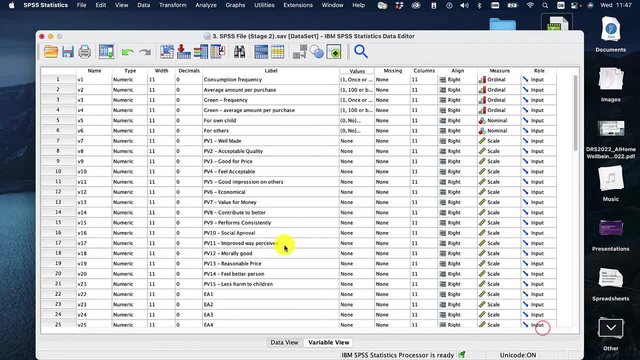 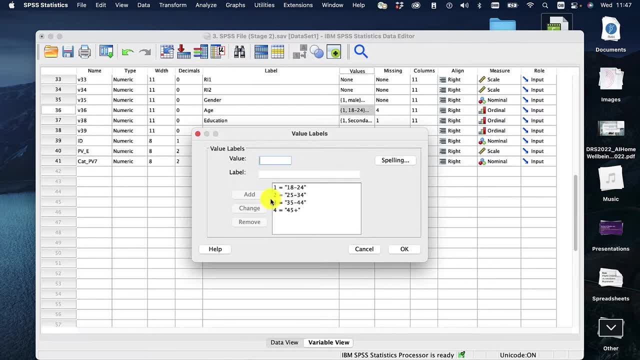 a variable which has more than 1 and 2.. So let's choose age: 1, 2,, 3, and 4.. So in that case I would choose maybe 2 and 3 or 1 and 4.. It's easy, but I'm going to choose gender because 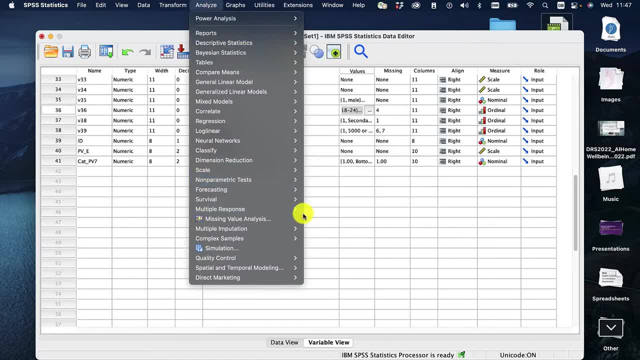 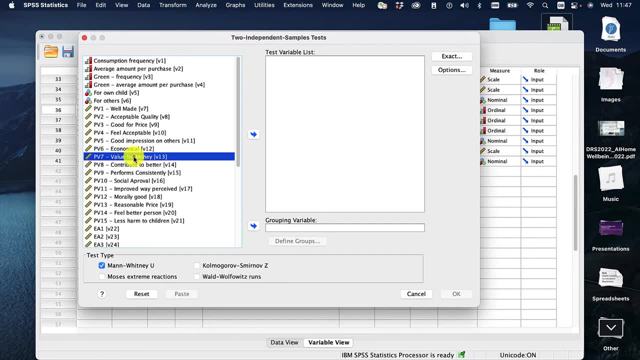 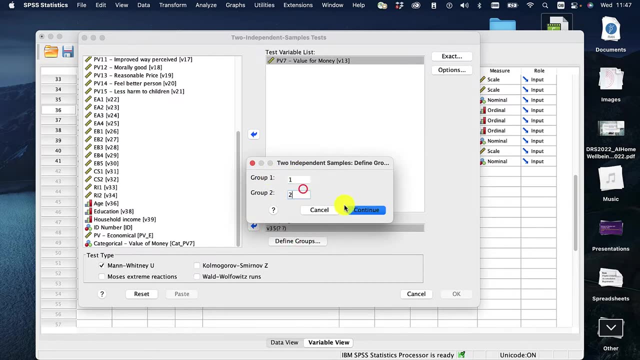 it just makes the example nice and simple. So non-parametric legacy dialogues and two independent samples. So pop this in again and value for money into the test variable and gender Grouping variable. define it as number 1 and number 2.. Click there. Now I've got a few things. 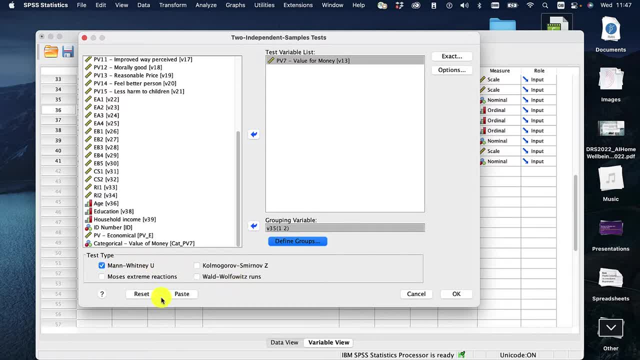 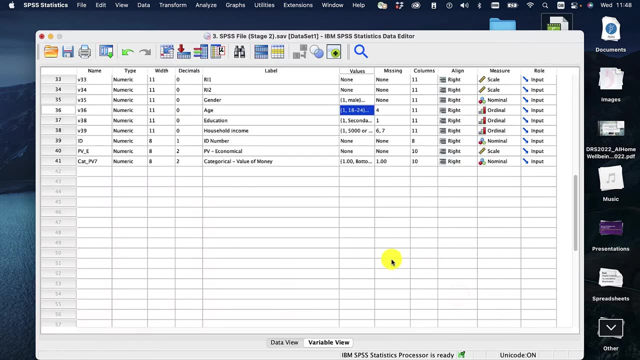 here I'm just going to go for Mann-Whitney uTest. There are things I can do, but everything's fine, The exact. I leave exactly where it is. Options: I make sure that I get descriptives and I want cases test by test. That is nice And click OK. This is going to give me everything I 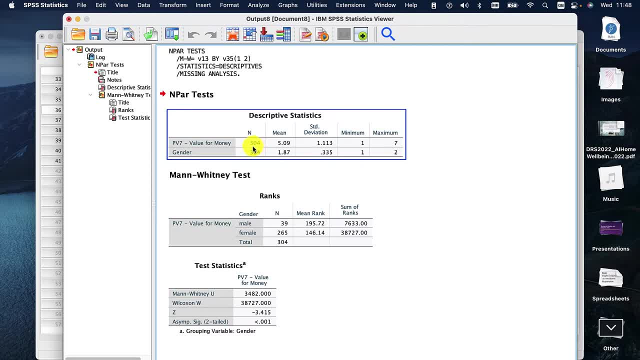 need. So first I can see I've got 304 people, which is very nice, And I've got a million people, So that's what this means for the whole thing. It doesn't really mean very much for us, So we can. 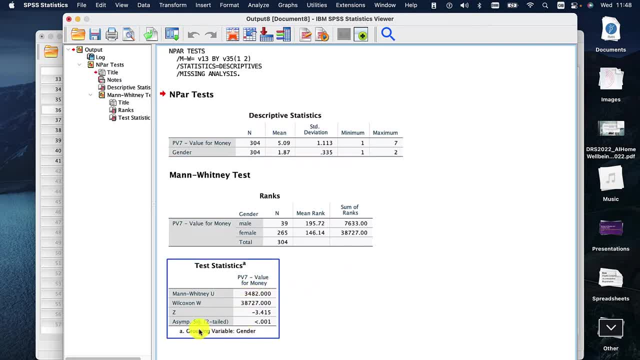 look at this and see that test statistics We have a significance of 0.001.. Actually it's less than 0.001.. So we've definitely got something going on here. There's a difference And we can see here that you know we've got 39 men and we've got 265 women. We know there's 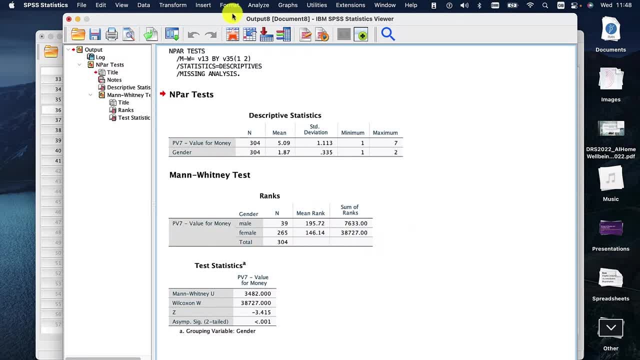 difference, but we don't know what that difference is. So for that we need to go and do a little bit more work. So we're going to go and do a little bit more work on the test. I'm going to go in here. 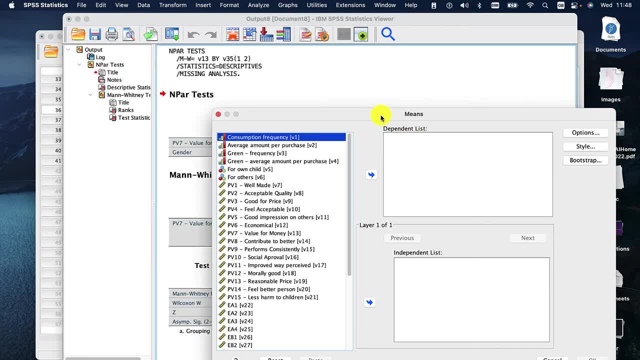 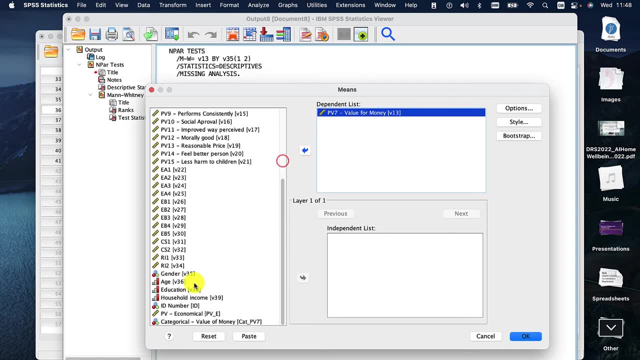 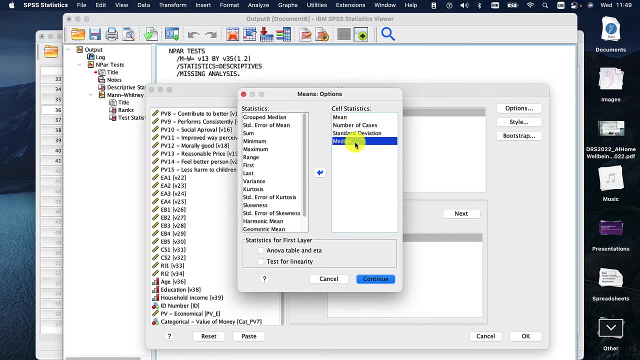 So analyze, compare means and means. For the pendant I'm going to chuck in value for money And the independent I'm putting as gender. Again, I can go to options. I want the median because that's what we use for non-parametrics.